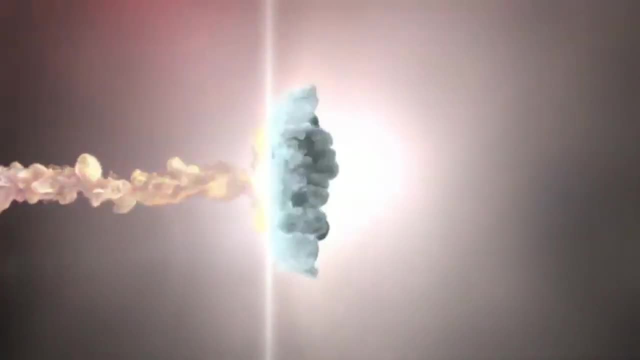 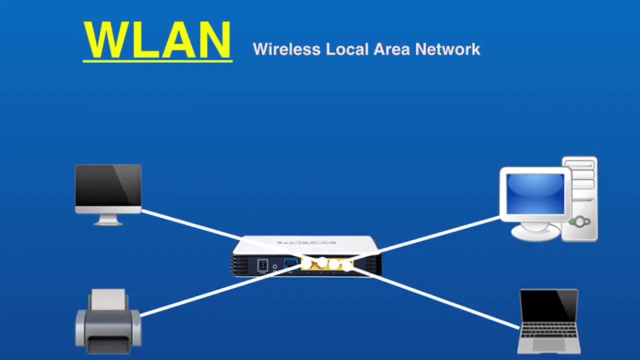 Hello everyone. Today we are going to talk about wireless local area network. A wireless local area network is a wireless computer network that connects to or more devices using wireless communication to form a local area network within a limited area, such as house, university or office. 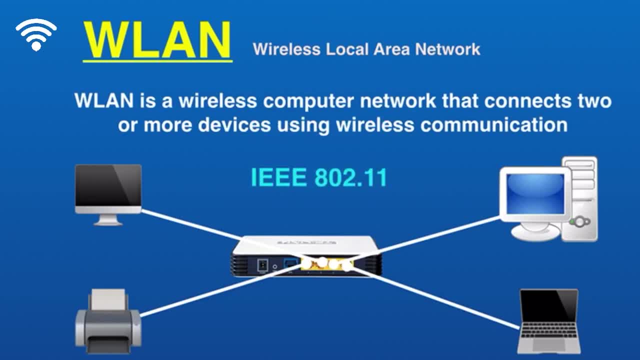 building. Most wireless LANs are based on IEEE 802.11 standards. Unlike a traditional wired local area network, in which devices communicate over ethernet cables, Devices on a wireless local area network communicate via Wi-Fi. Wireless local area network uses high frequency radio waves. 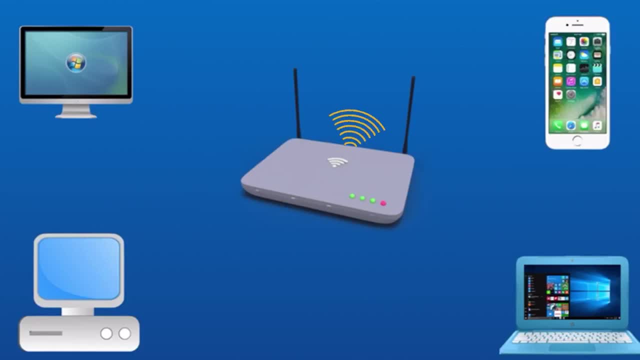 While a wireless local area network may look different from a traditional local area network, it functions the same. New devices are typically added and configured using dynamic host configuration protocol. They can communicate with other devices on the network the same way they would on a wired network. 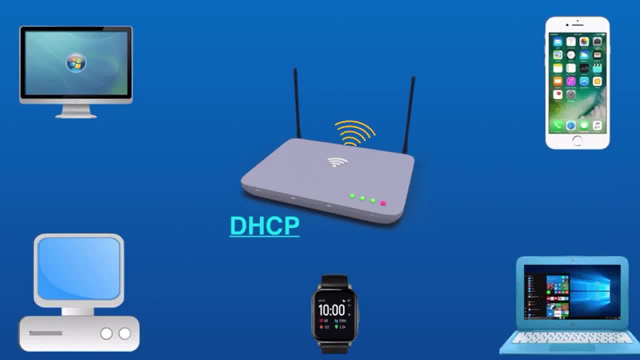 The primary difference is how the data is transmitted. In a local area network, data is transmitted over physical cables in a series of ethernet packets. In a wireless local area network, packets are transmitted over the air. Packets contain instructions and MAC addresses of the connected devices that enable routing to the intended location. 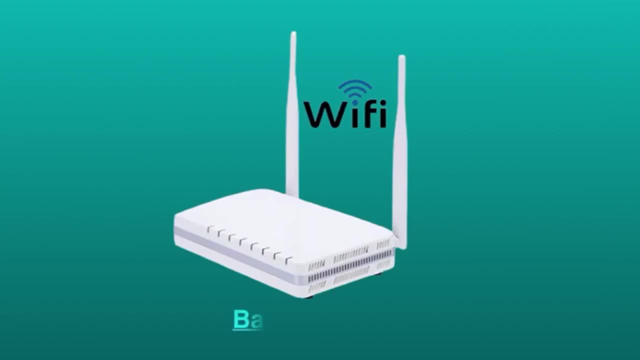 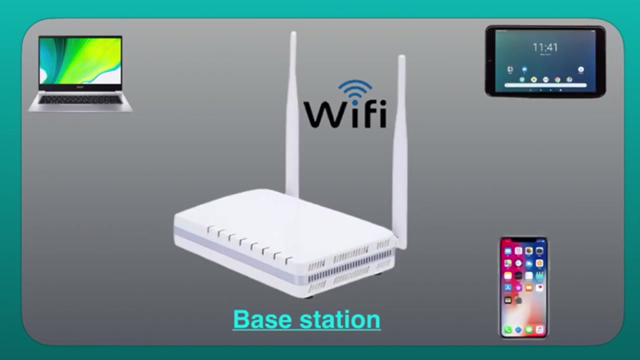 Nowadays, most of the routers are coming wireless. A wireless router serves as a base station, providing wireless connections to any Wi-Fi-enabled devices within the range of wireless routers. This includes laptops, tablets, smartphones and other wireless devices such as smart appliances and smart home controllers. 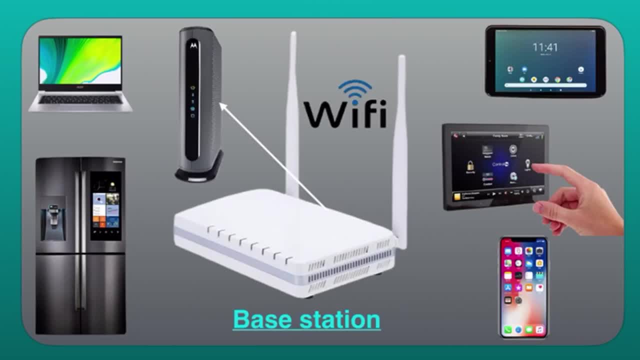 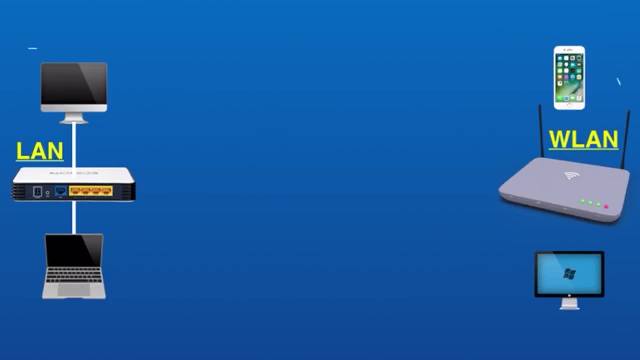 Wireless routers often connect to a cable modem or other internet-connected device to provide internet access to connected devices. Local area network and wireless local area network can be merged using a bridge that connects the two networks. Wireless routers that include ethernet ports can automatically combine wired and wireless devices into the same network.